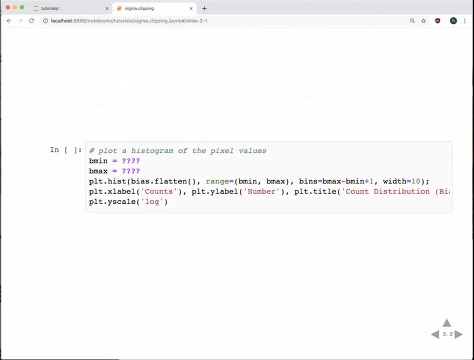 And now We have that data loaded in, We can plot a histogram of it just to see what the distribution of values looks like. So we need to pick how we're going to do this histogram. We're just going to take all the values and send it to plot dot hist. 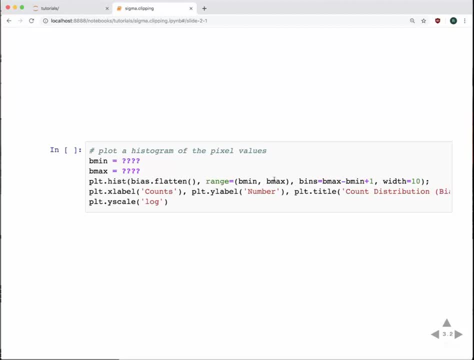 And we can tell what range we want it to be plotted over, what the minimum and maximum values of the range are going to be and then how many bins we're going to have. So to set the minimum and maximum range, it makes sense to just take the minimum and maximum values of our bias. 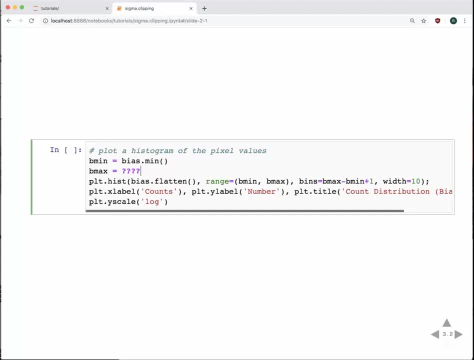 So we'll take bias, min and bias, And then we'll plot this up And then we'll have one bin for each data value. So we're going to have values that go from, say, 450 to 550.. And so we'll have a bin at 450, 451, 452, et cetera, falling this way. 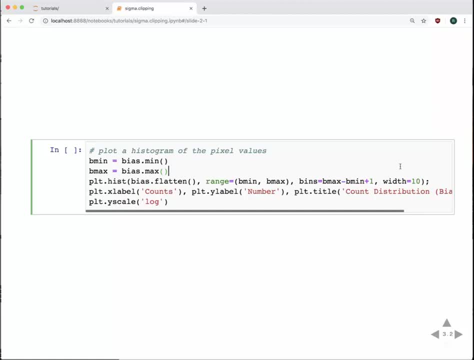 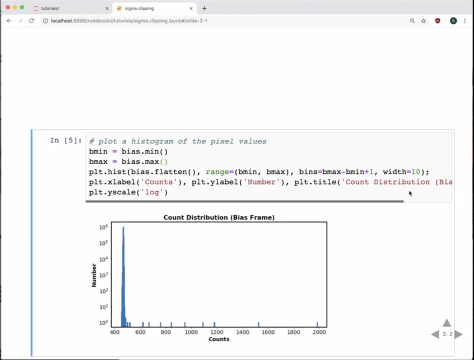 And with here is just going to make those bins wider so that the plotting appear wider. I'll show you so that we can actually take a look at that. So we're going to take a look at that. We're going to take a look on the screen here and actually see them. 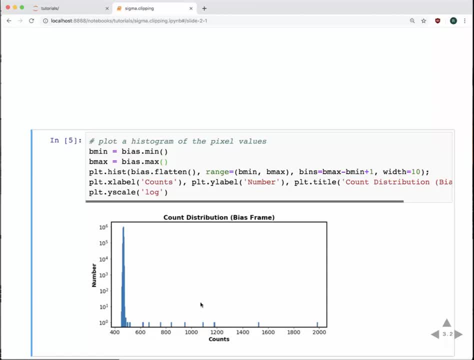 So these guys are going to be just thicker because of that width keyword. All right, So here's the distribution we have from our bias frame. You can see this is on a log scale here, So the vast majority of pixels are located around 450.. 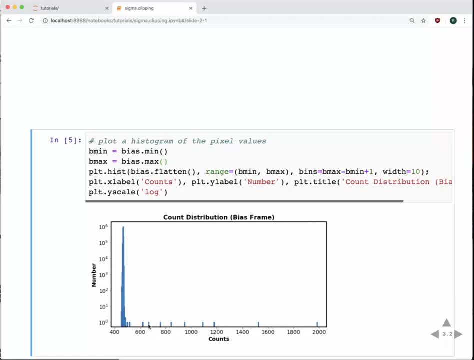 And then there are a few pixels- and this is just one- in each one of these upper bins here that are scattered up all the way to almost 2,000.. All right, So you can look at this pretty quickly and say this is the distribution of bias values that I should have. 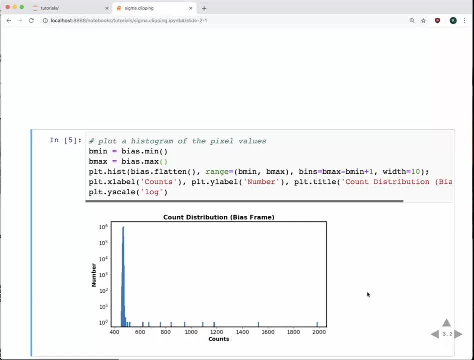 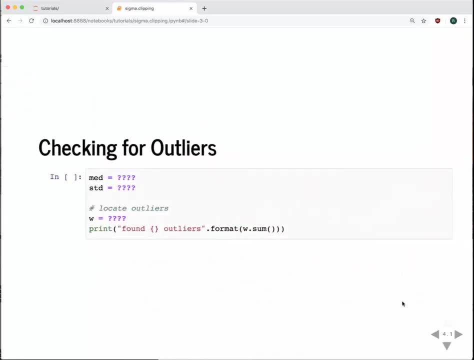 And then I have some outlier pixels on top of that. So what we're going to do now is figure out how to identify these outlier pixels and ultimately reject them. All right, So one thing you can do to check for outliers is you can figure out what the median value of your sample is. 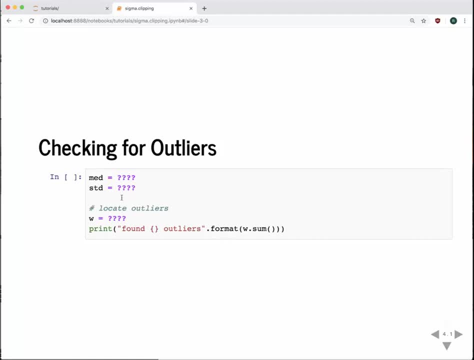 or what you think your median value of your sample should be and what its standard deviation should be. And then you look for pixel values that are some number of standard deviations above or below that expected- those expected, All right. And then you look for pixel values that are some number of standard deviations above or below those expected limits. 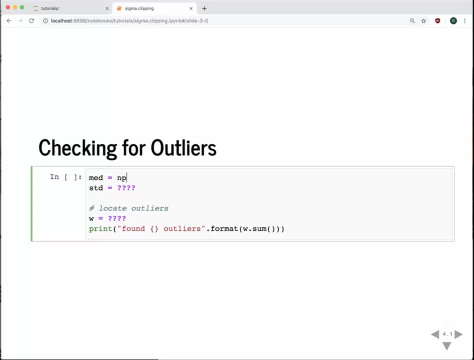 So we could take the numpy mean of our bias frame. But since we do have those outliers, if you think about it for a moment, what are those outliers going to do? Well, they're all on one side, So they're actually going to raise that mean value a little bit higher than it should be. 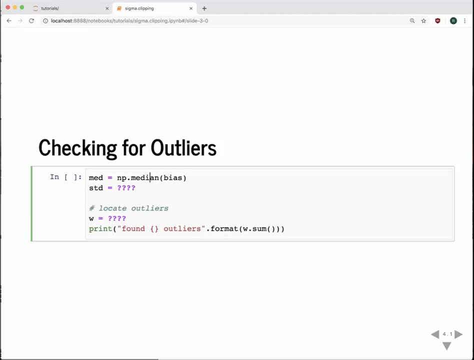 So, instead of taking the mean, we can take the median, And this is a little bit more robust when you have outliers. So remember the median value is just the median, It's the value that's right in the middle of the distribution. 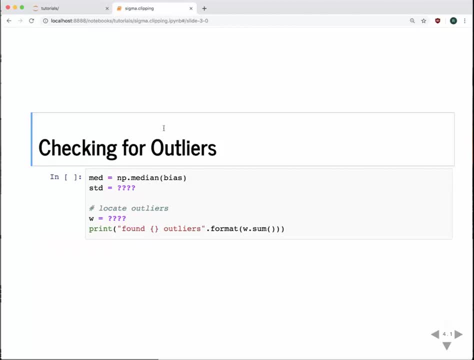 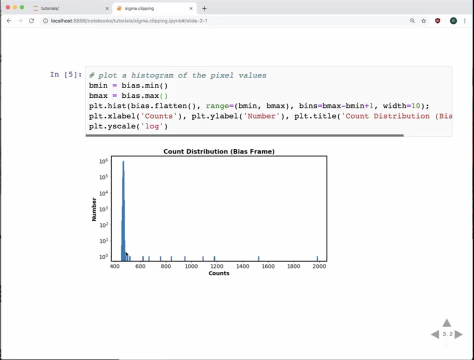 So half the values are below and half the values are above. Now we saw in this plot that we have a few values- This is maybe 10 values that are much greater than our expected mean value here, But we have a whole pixel. 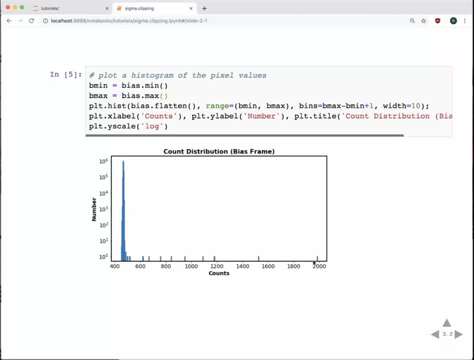 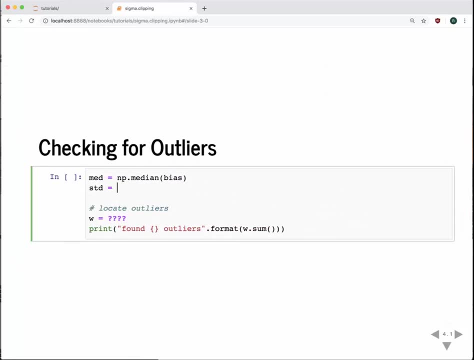 We have millions of bins here, So a few data points are not going to affect the median. And then, on top of this, we're going to take the standard deviation and we'll see how we can deal with the effects of those outliers and the standard deviation in a minute. 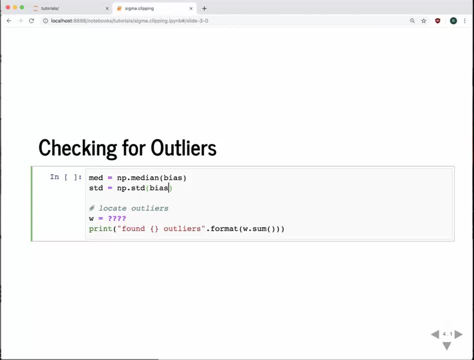 But for now we'll just take numpy standard deviation of the bias- And we don't have to do this since we have so many data points. But just to be exact, we'll specify delta degrees of freedom of 1.. OK, So that'll give us our median value for our image, which remember. 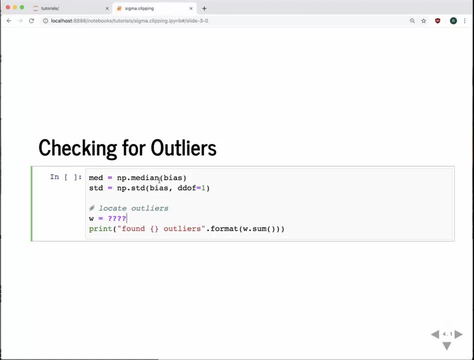 if you have a Gaussian distribution, the mean and the median are equal, So the median value here is actually a good representation of the mean For that Gaussian distribution. So now we just need to identify which are our outliers, And the way that we can do this is we can take our bias values. 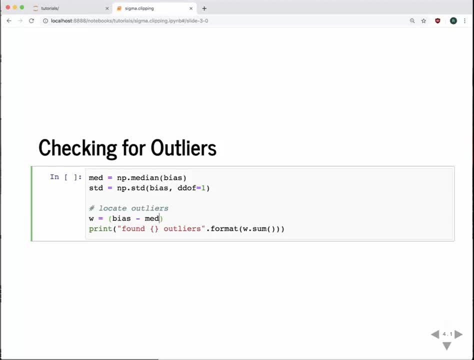 and we can subtract off that median value And that'll give us the difference, And what we care about really is just the absolute difference. We'll use numpy abs to get the absolute difference between the bias values, all those millions of values, and the median value we calculated. 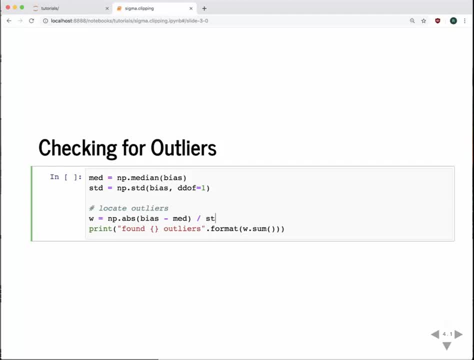 And then we're going to see how many standard deviations off those pixels are, And then, finally, we're going to ask how many of those are some number of sigma away from the mean. So we'll say 5 sigma in this case. 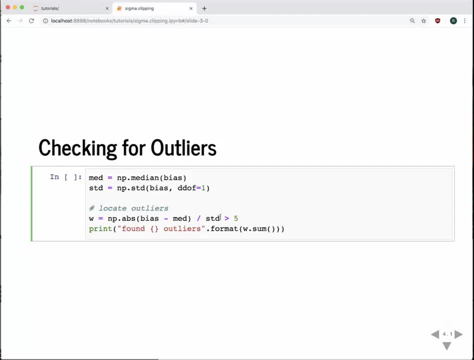 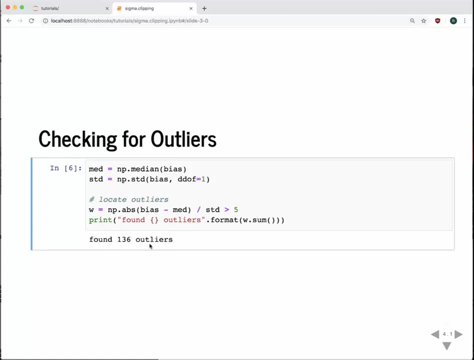 So we're going to find how many pixels are 5 sigma away from above or below from the median value, And in this case there's 136 pixels that we're going to consider outliers. We can just quickly plot what this looks like. 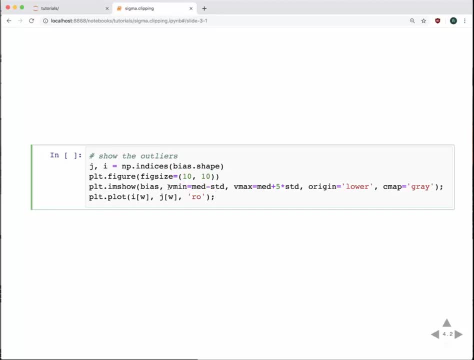 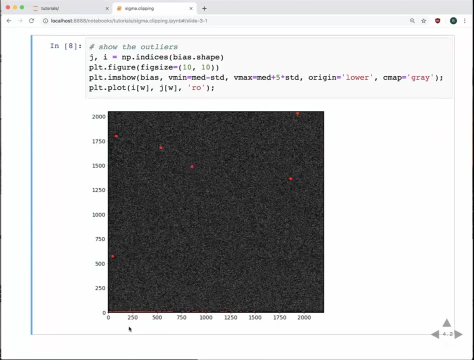 Just to give some graphical representation of what's going on here. So I'm just going to bring up this figure and explain what's going on. So what we're doing is we're identifying which of these pixels are bad and we're marking them with little red circles. 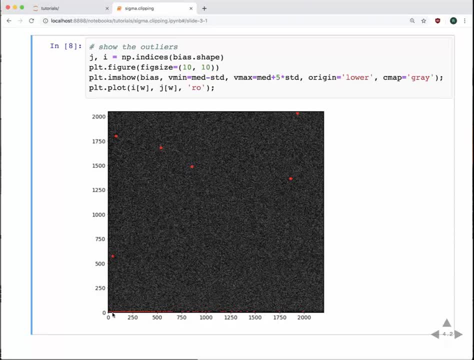 So on the bottom of the image here we have a whole bunch of bad pixels on the bottom here, And then, scattered above, there's just a handful of pixels that are deviant as well. So this down here, just so you know, is a feature of our bias. 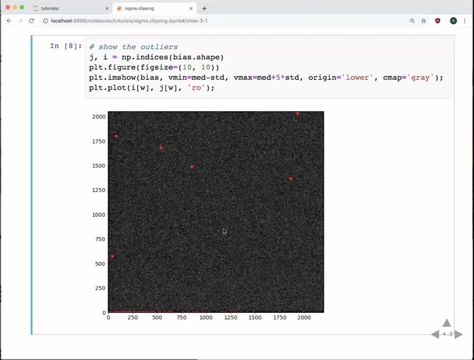 And it turns out that the values in this first couple of columns here are a little bit off from the rest of the image And these pixels up here actually represent most likely cosmic ray events. All right, so we saw that we have these outliers. 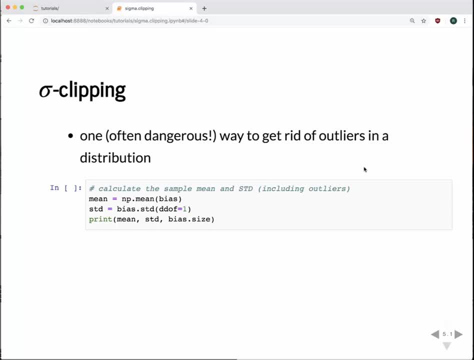 And we were talking about how the mean and median values might be discrepant because of that. But the outliers also have an effect on the standard deviation, So we're going to take a look at that now. So first we're just going to calculate again just the mean, not the median. 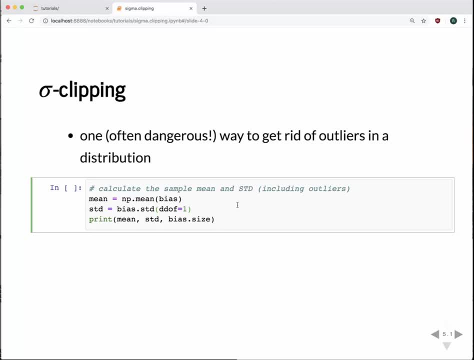 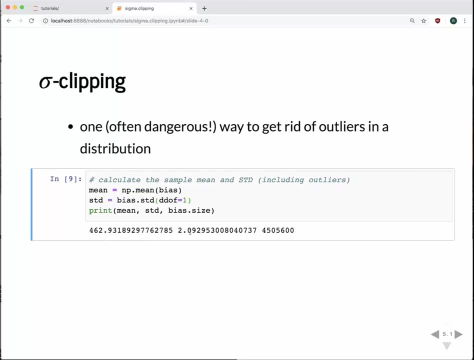 but the mean value of our sample And the standard deviation, And we'll just print those out. And so here's: the mean value is 462.93.. And standard deviation is about 2.1.. And this is the total number of pixels we have in our image. 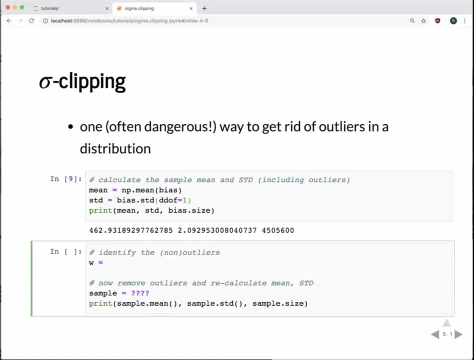 And again there's over 4 million pixels. We get a lot. So now what we want to do is actually identify the pixels that are not outliers, And we've already got a variable that we could use to do that, But I'm going to define it again and just do it slightly different. 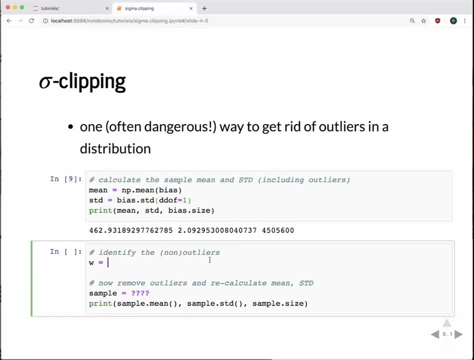 So I'm going to have a new w here which, instead of being the outliers, is the non-outliers, And so we can just do what we did before. Take a numpy absolute value of the. we'll do the mean value in this time. 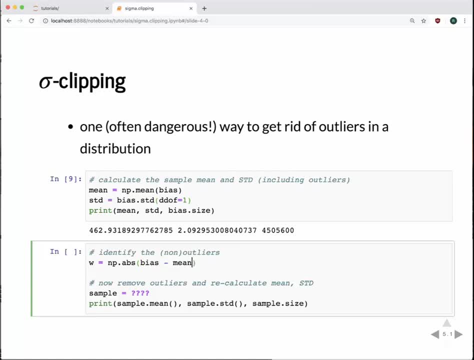 So the bias minus the mean, And we're going to ask which of these pixels are less than 5 times the standard deviation. And then what we can do is we can take our bias sample And we can just take a slice of it that corresponds to the values that are with us. 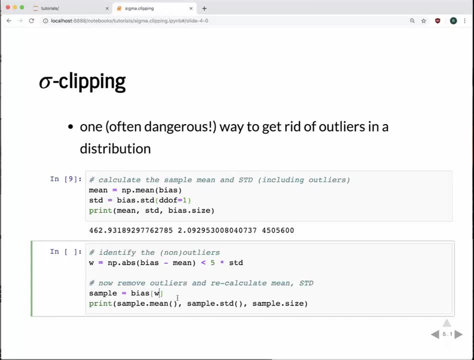 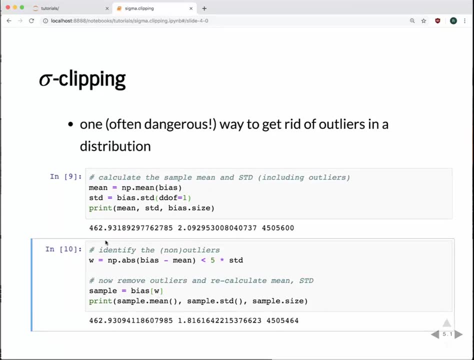 Within 5 sigma. So we're not using outliers, We're just using the ones that are within the expected distribution. If I run this, we can see what the mean and standard deviation of that is, And so for the, the mean value actually didn't change that much: 460.93,- pretty much like. 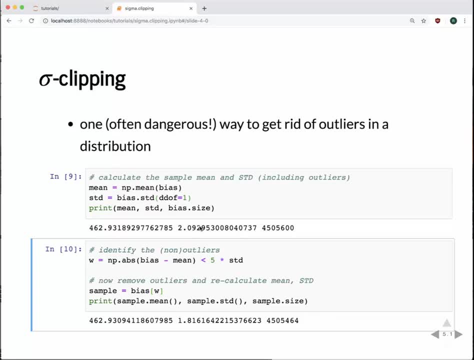 we had before. It's a very small change, But you'll notice that the standard deviation actually changes quite significantly. So even though we just had 136 pixels out of 4 million- that are outliers- They make a significant difference. They make a significant change on the standard deviation. 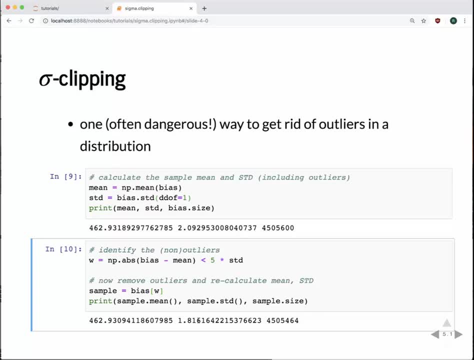 And that's how the that has to do with how the standard deviation is defined. So this is very important to note And the result is that when we did that- that clipping calculation- originally, we removed the points that we thought were 5 sigma greater than the mean. 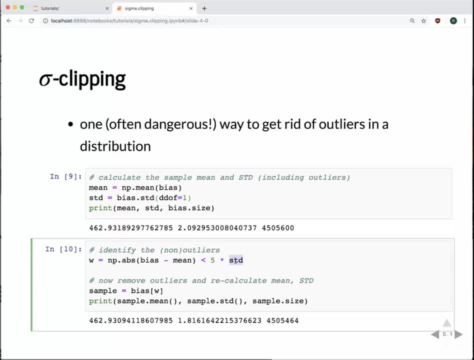 We were using the wrong sigma. The sigma we actually used should have been a little bit smaller. So we've got to think now: how can we deal with this? What is a more robust way to actually figure out what that standard deviation is? 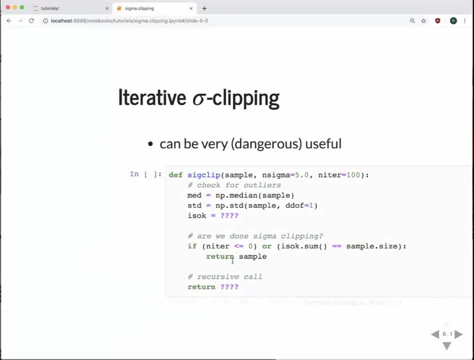 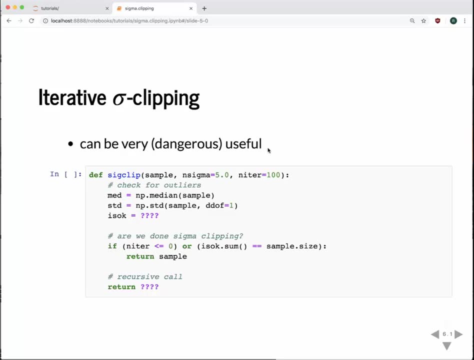 What do we need to do about that? standard deviation and mean are when we have outliers. So the solution is often to do what's called iterative sigma clipping. Those can be very useful to do, but it is actually somewhat dangerous. you've got to. 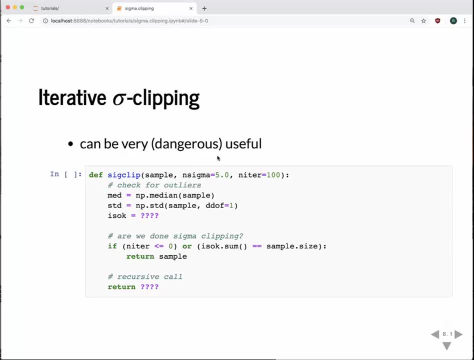 be careful that you're not cooking your data here, that you're not over clipping your data. So what we're going to do is we're going to find a little function that will actually go through and calculate the mean and standard deviation And then figure out where the outliers are. 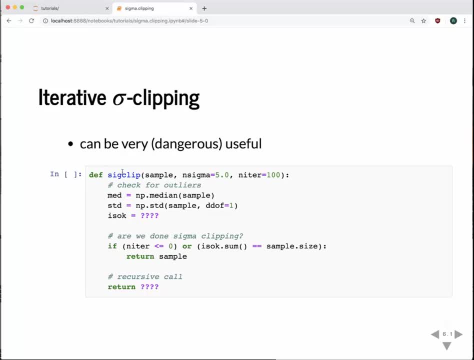 And after we've done that, we'll reject the outliers and then we'll call the function again to do the clipping again, And we'll keep doing that until we've done maybe 100 iterations or however many we want, or if we stop removing data points. 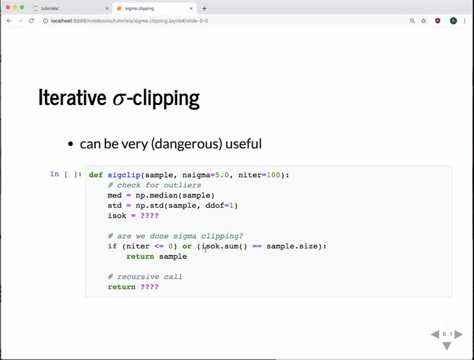 So if we get to a point when we try and clip out data points and every pixel passes, we know we don't have to do it anymore. All right, so we're going to again start by using the median. That's a good estimator of the mean if you have a Gaussian distribution. 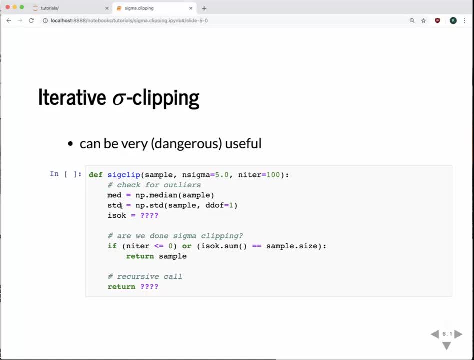 It's more robust. We're going to use standard deviation of that sample and then we're going to figure out which pixels are the ones that we want to use, And I'll just write this in one slightly different way that I've done already. 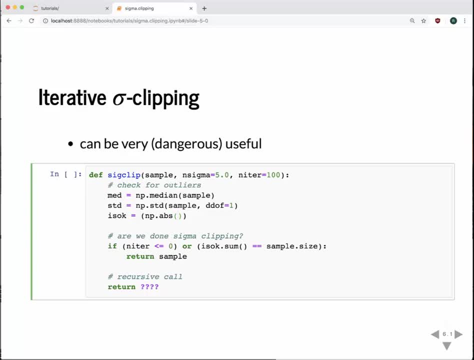 So again, we're going to use numpy- absolute value of our sample minus our med value, our median value, and then we're going to divide that by our standard deviation, And then we're going to take this whole thing and we're going 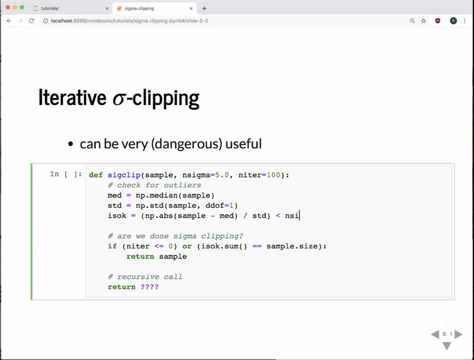 to add that to our median. And then we're going to ask: is it less than some number of sigma? And by default we're going to have n sigma set to 5, but we can change this to 3 or whatever. 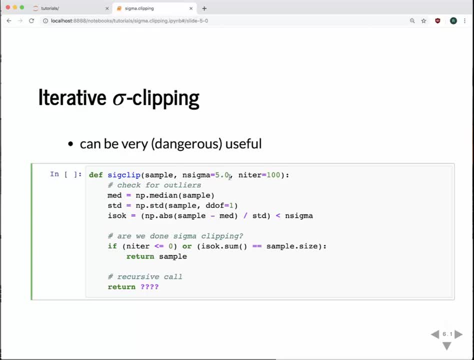 So we can reject pixels that are 5 sigma or 3 or 4 or whatever we put here. Okay, so once we've done that, then we can go through and we can say: are we all done Or should we just return this sample of values that we've found? 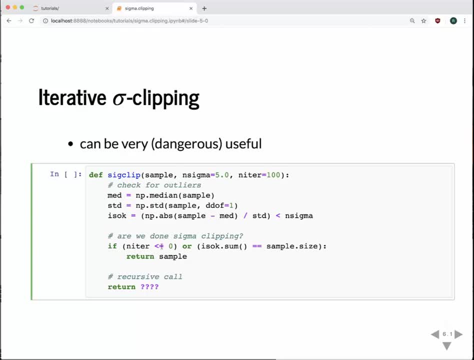 So we do that by checking if we still have iterations left to compute and see if did we return it Or did we reject any points this time. If we did reject some points and there's more iterations left, then we can actually just return a recursive call to sigma clip. 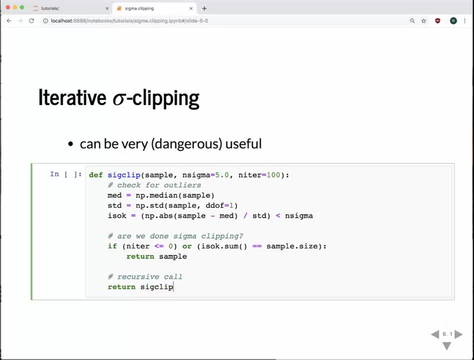 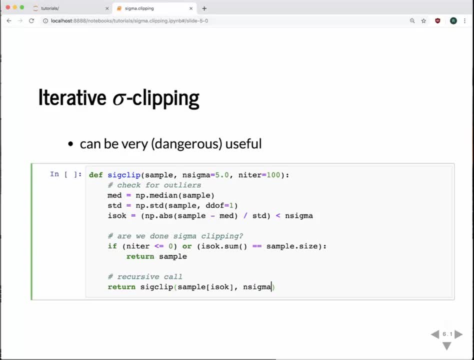 And we'll pass the n sigma And we'll pass the n sigma. That's the constraint on where we're going to define that sigma clipping. And then we're going to take the n iter we had and we're going to subtract 1.. 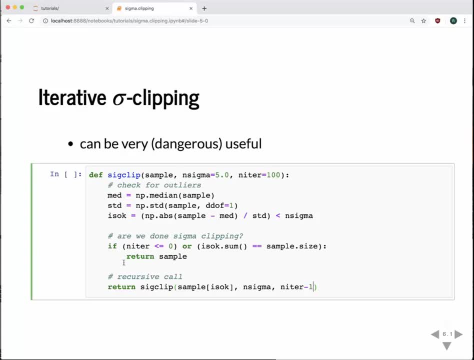 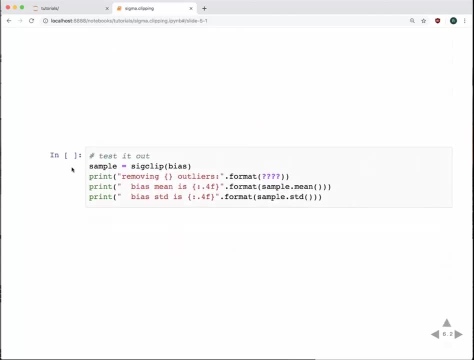 So just every time we run this, we'll subtract 1 from n iter. So when it gets down to 0, then we'll stop. Okay, so we have our function defined now And we can try and use it. We'll take our sample. 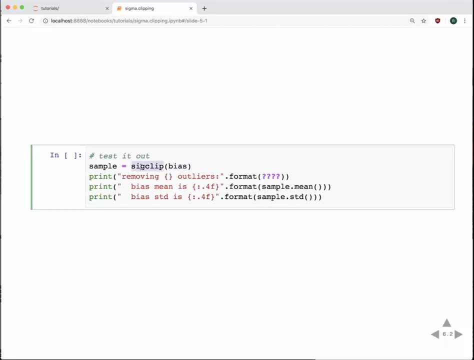 Well, sorry, we'll take our bias sample and we'll run pass that to sig clip, It'll iteratively remove And we'll finally return that sample after it's done as many iterations as it can or until it's no longer removing any pixels. 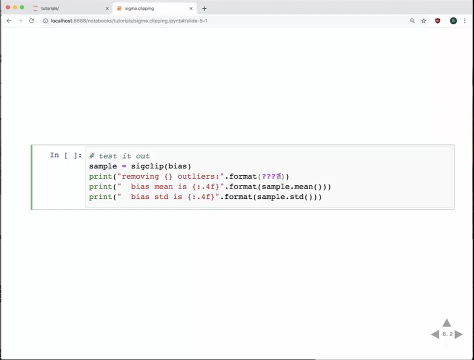 And then we'll see how many pixels it removed and what the bias mean, value and standard deviation is. So to figure out how many pixels we have removed, we'll take the size of the, the original size of the bias, and just subtract off the size of our sample. 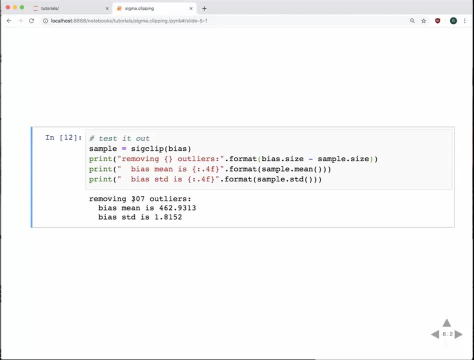 So if I run this, We found that we've now removed 307 outliers through all of our iter iterations, The biases. the mean value is close to what we had before, 462.93.. And the standard deviation now has dropped slightly more. 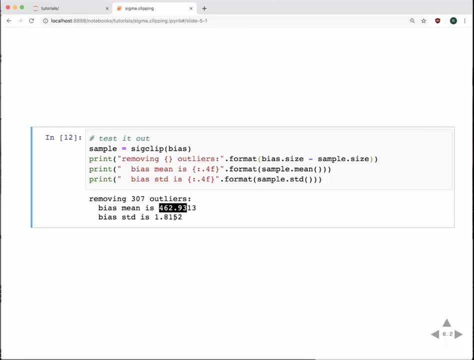 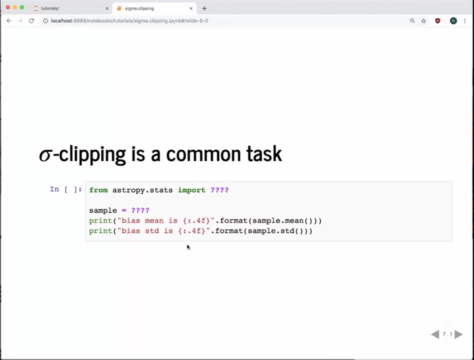 So it's now 1.815.. So slightly below what it was before. Sigma clipping is a very common task and it's actually built right into AstroPy. So if you go to AstroPy stats, there is a function called sigma Clip and we can run sigma clip very similar to the function that we defined, our sig clip. 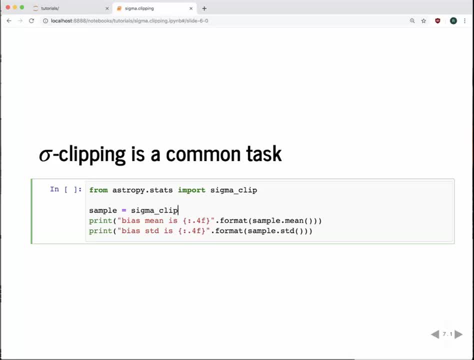 Just by running it on our bias frame. Now the version of sigma clip by default actually uses a value of n, sigma of 3.. So if we want to change that to match what we did before we're going to do, sigma equals 5.. 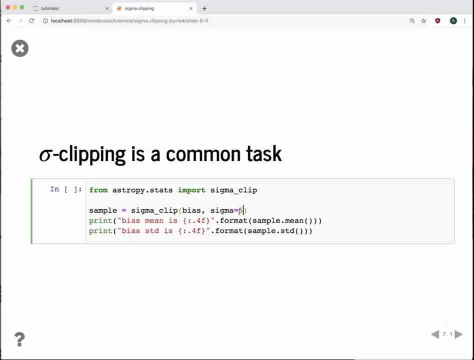 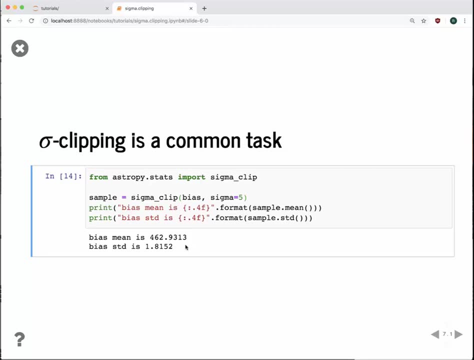 So if we run this with a threshold of 5 sigma, it'll run through and we'll turn numbers. that should look very familiar because it's basically doing. it is doing exactly what we've coded up already. So, as I mentioned, the default value is actually 3.. 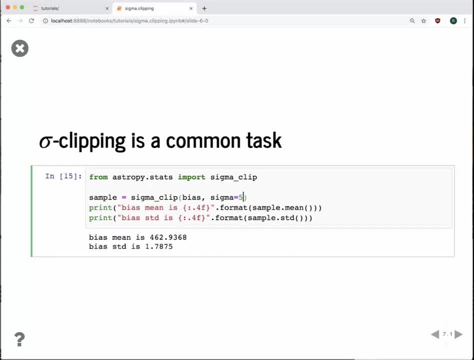 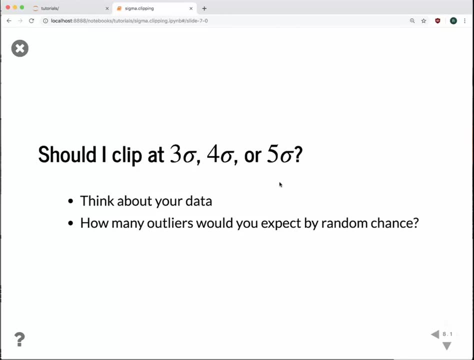 They do 3 sigma by default, So why did I pick 5?? Why shouldn't we do 3 in this case? We should think about this: How do I know how many sigma I should clip my data at? And this is an important question. 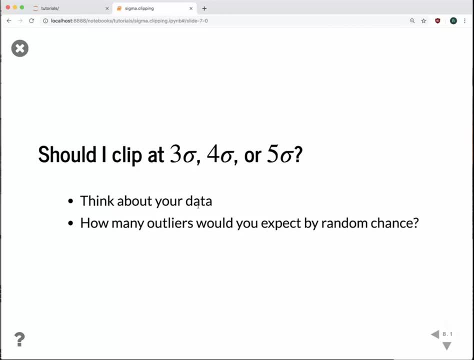 And you really have to think about What your data are. how are they distributed, what is the range of values- and you should ideally know something about your outlier population as well- And if you know something about the data you have and the distribution you expect to get. 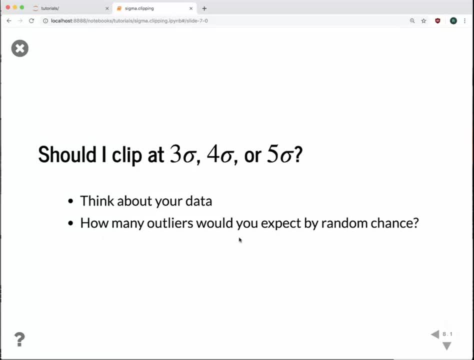 then you can actually predict how many outliers you expect to get by random chance. And then you should set your sigma clipping so that you don't remove any real data points. So to figure out if we should do 3,, 4, or 5 sigma clipping, we're going to start by figuring. 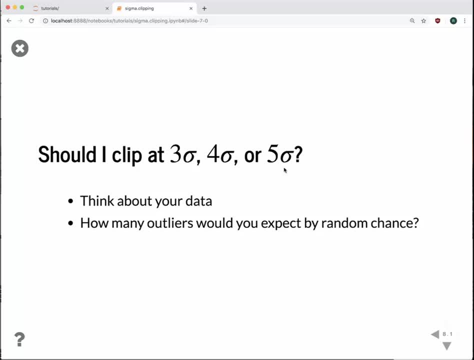 out how many Um Pixels in our bias image. we would expect, just naturally, to be 3,, 4, or 5 sigma, even if there was no outlier population. So the way we're going to do this is we're actually going to assume we have a Gaussian. 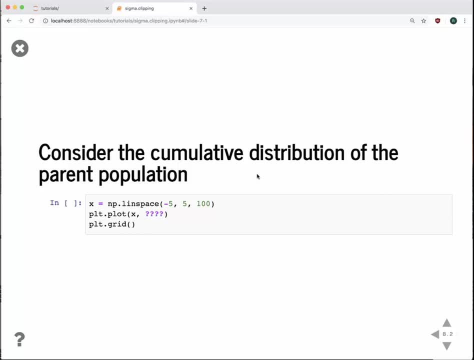 distribution, that the true bias distribution is Gaussian, And then we can predict how many 5 sigma outliers should we have. So to show you how we can do this, I'm just going to start by defining a bunch of x values, from minus 5 to 5.. 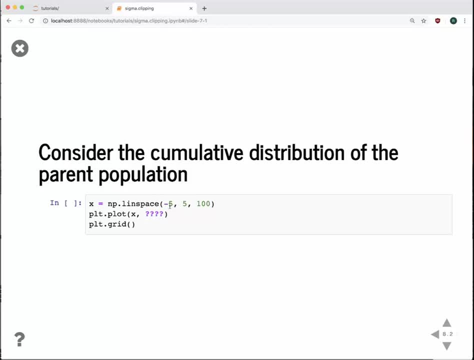 This is going to represent how many sigma away from the mean value we are Sigma below or 5 sigma above. And then we're going to plot those x values and we're going to plot the cumulative distribution of a Gaussian. So this is in psi, pi stats, and we're going to use the norm for our normal distribution. 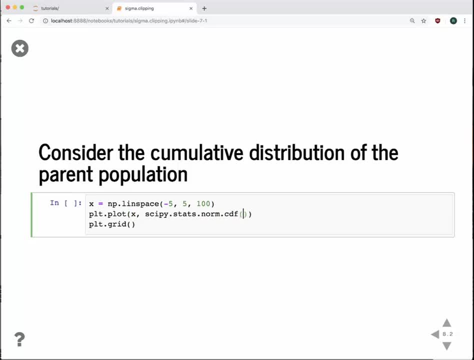 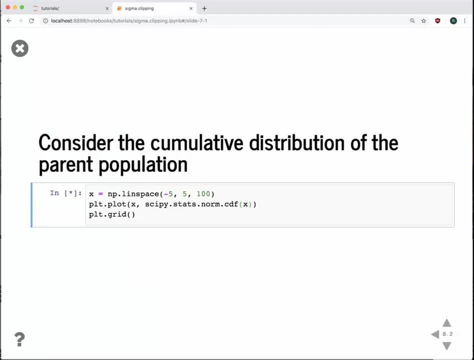 And we're going to plot the CDF, the cumulative distribution function, And we're going to plot it for each one of these x values. So each x value, we're going to have the cumulative distribution to that point and we'll plot this up and talk about it. 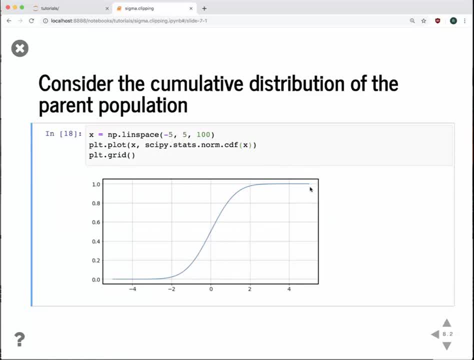 So, again, this is a cumulative distribution. This is a cumulative distribution of a Gaussian distribution And, at any value, if you pick this point right here, it's telling you the fraction of the population that is less than or equal to that point. 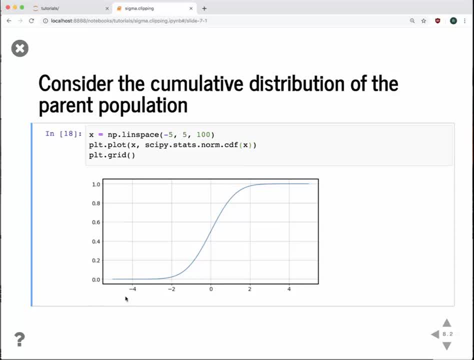 So this is the fraction that is less than or equal to some number of sigma away from the mean value. So by default, the mean value here is actually zero. That's our Gaussian mean. It's zero, And you can see that 50% of the data points. 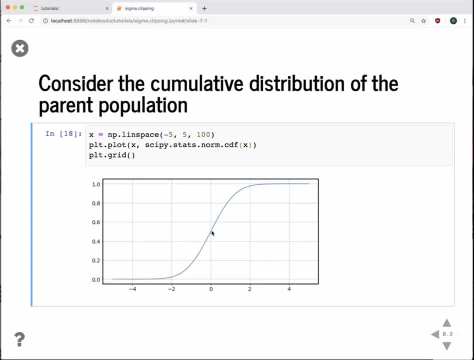 Are below zero. That's what you expect for Gaussian And the Gaussian symmetric. So again, 50% are above zero. Now, as you move one sigma or two sigma away from your mean, you can say how many points are below, say, two sigma below the mean right. 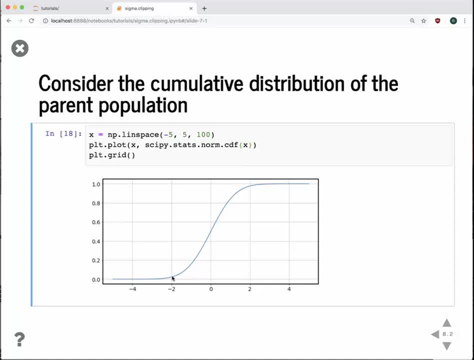 So if I go to, if I look at all the points that are two sigma below the mean, I can see the fractions. a tiny fraction, just a few percent of all the data points are two sigma or less than zero. Uh, Most of the data points are two sigma above the distribution or less. 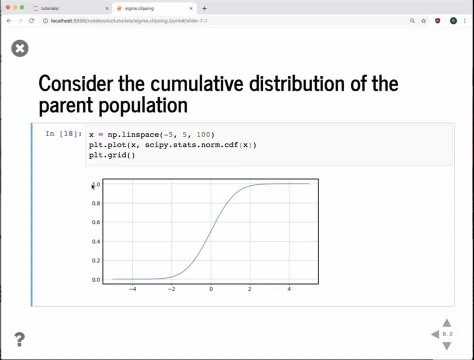 So, since this is just giving us the fraction of our sample points, that should be two sigma or one sigma or four sigma below or above our distribution. uh, what we can look at is say: how many data points do we actually have, and then we can predict how many of them. 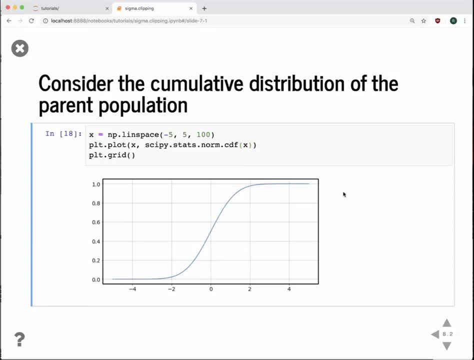 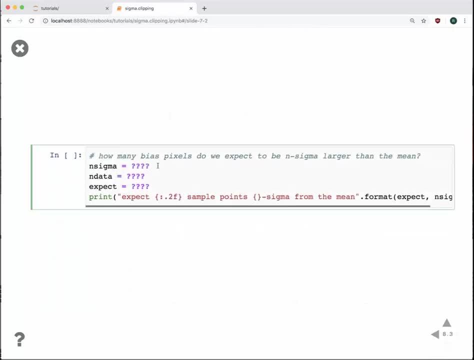 should be, you know, four sigma below or four sigma above, uh, the mean value. Okay, So before we actually get to that bias frame, let's just say we had a smaller sample. Uh, so let's say we had maybe just 50 data points. 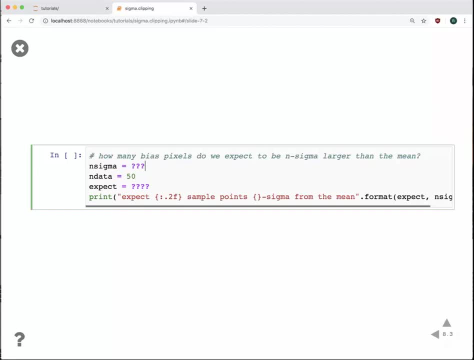 If we had 50 data points and we want to know how many three sigma outliers, what do we expect? Well, how do we calculate this? Well, we can again use our SciPy stats. CDF, The norm, uh, CDF. 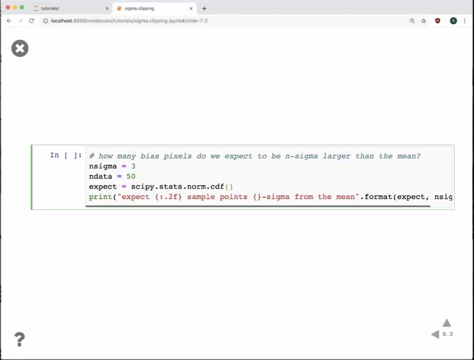 And we can predict. Okay. Okay, So we can pass it in sigma and that'll tell us, uh, the number of values that are below n sigma. It's not quite what we want. We want to know the number of outliers we have, so we want one minus this. 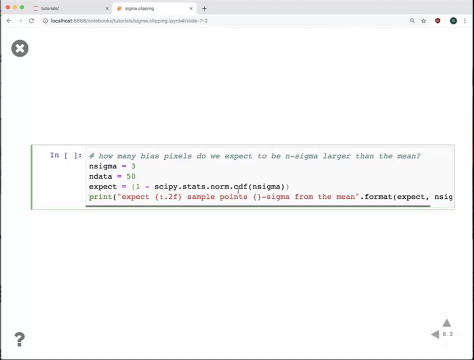 We only care if a given data point is three sigma away from the distribution. We don't care if it's above or below, so we don't care about the sign and that means half of the values are going to be less than three sigma. half of the values are going to be. 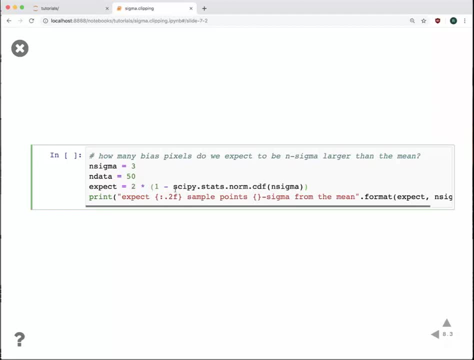 greater than sigma. So we're going to double count here Each one of these, And then we're going to multiply by the number of data points we have in data And if we print out this, this will tell us that if we have 50 data points, we only expect. 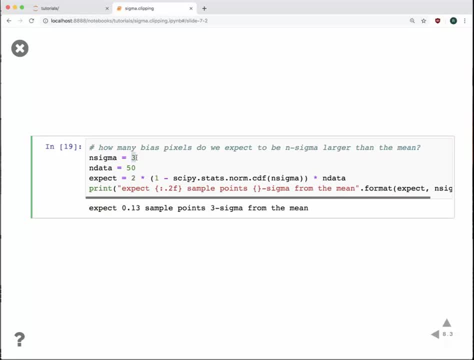 .1 outliers at the three sigma level Only .1.. So basically, if you, if you had a sample of 50 data points and you clipped out everything that was three sigma away, you would expect that none of your data are actually getting.